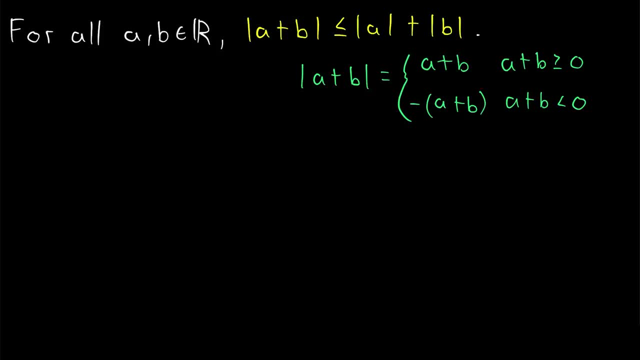 both a plus b and negative. a plus b must always be less than or equal to the absolute value of a plus the absolute value of b. that will complete the proof. We want to begin by noticing four obvious inequalities. Certainly, a is less than or equal to the absolute value of a, and negative a. 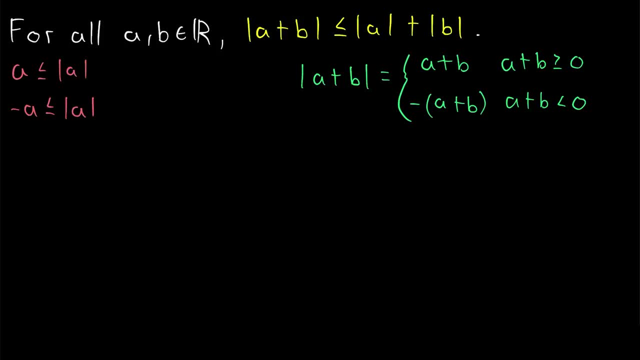 is less than or equal to the absolute value of a. This is because a and the absolute value of a have the same magnitude, and if a is negative, it will be less than its absolute value. Similarly, we know that b must be less than or equal to 0.. If a is negative, it will be less than or equal to. 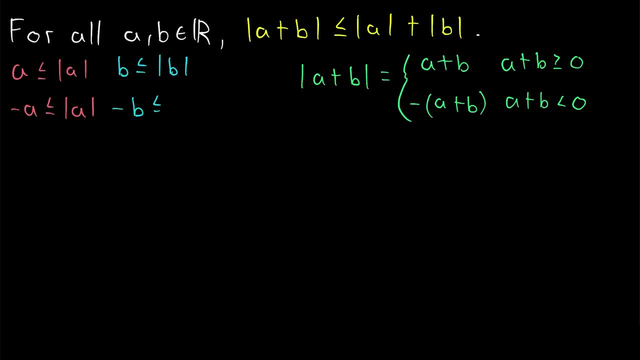 the absolute value of b and negative b is less than or equal to the absolute value of b. Again, the only potential change the absolute value function might make is making the number positive, and a negative is always less than a positive. Then we can easily work our way through to our 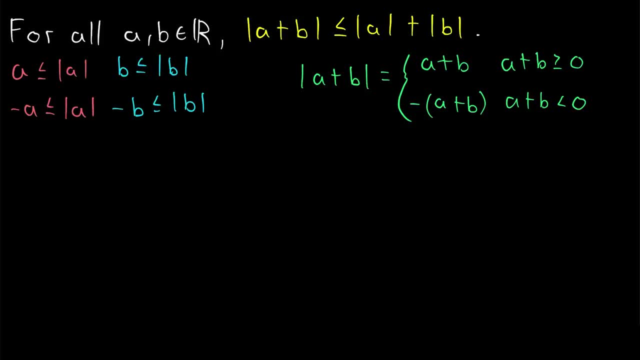 desired conclusion. Let's start with a plus b. What do we know about a plus b? Well, certainly, it's less than or equal to the absolute value of a plus the absolute value of b, Since we just remarked that a is less than or equal to its absolute value and b is less than or equal to its. 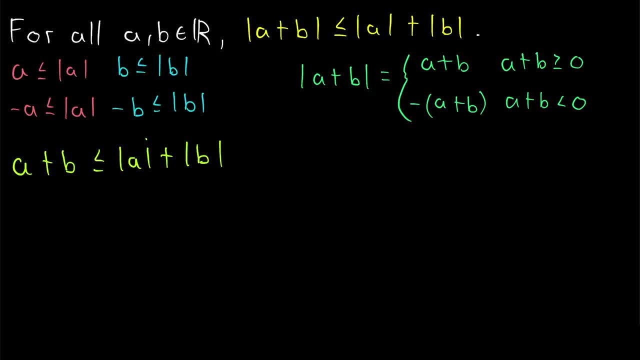 absolute value. So if we replace them both with bigger numbers, we get a bigger number. That's the inequality we were looking for. so we can stop there and move on to negative a plus b. So what do we know about negative a plus b? Well, distributing the negative, it's equal to negative a. 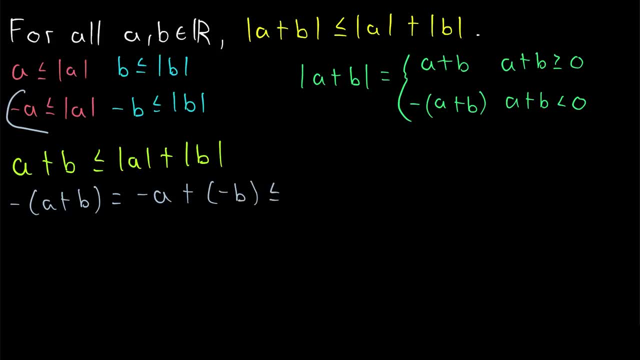 plus negative b. And we just went over how negative a is less than or equal to the absolute value of a plus the absolute value of b. So if we replace them both by greater numbers then we get a greater number. So negative a plus negative b is less than or equal to the absolute value of a plus. 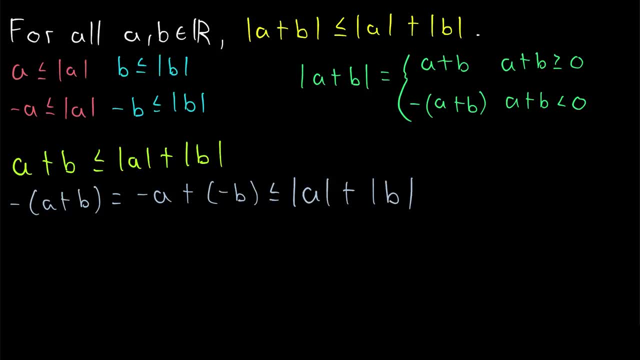 the absolute value of b. We could have also done this in smaller steps. if that makes you more comfortable, We could replace negative a with the absolute value of a and leave negative b unchanged at first. This inequality is certainly true, since we replaced negative a with a number that's greater.